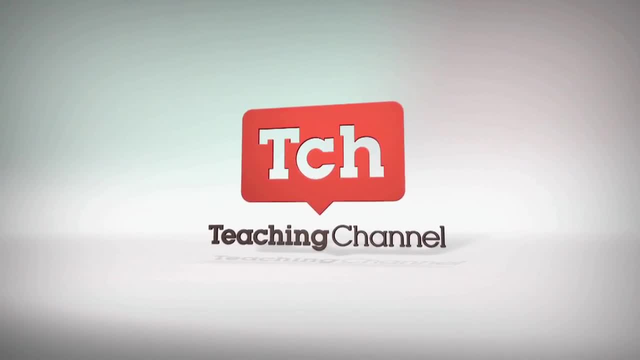 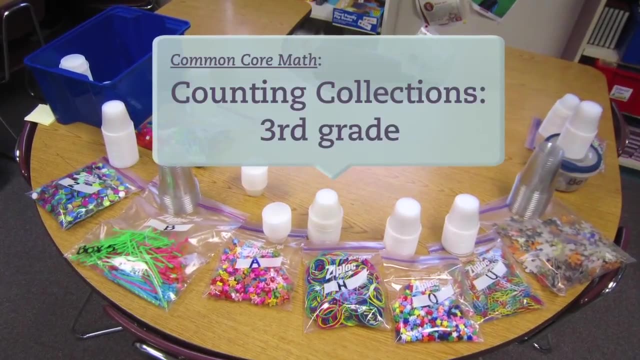 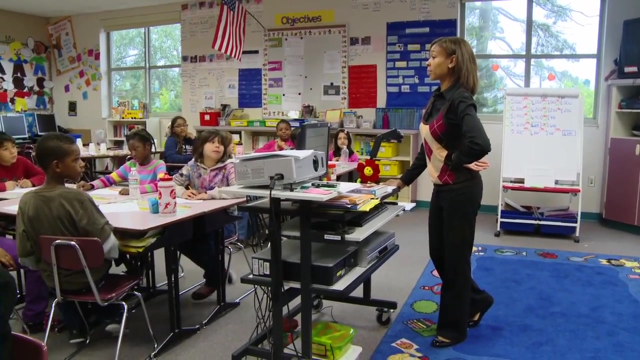 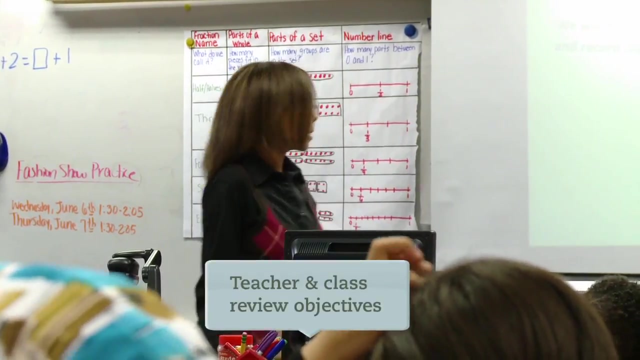 We're going to do a counting collection today, and each one of you are going to get a group of objects, and so you'll be counting those. So we're going to read the objectives together. Okay, ready, Begin. We will estimate the number of objects in a collection. 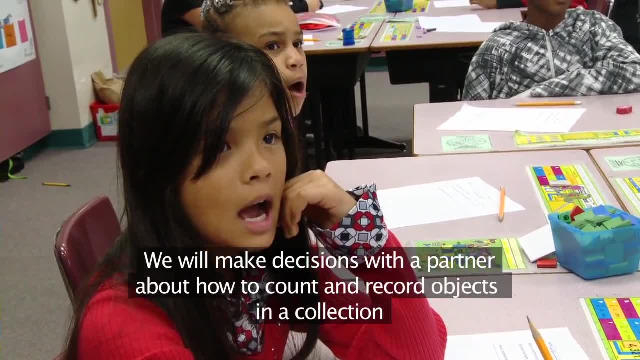 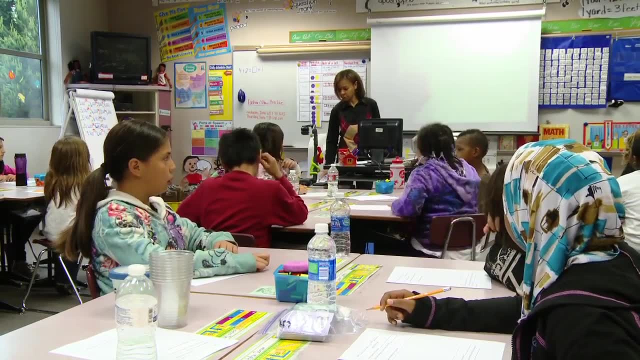 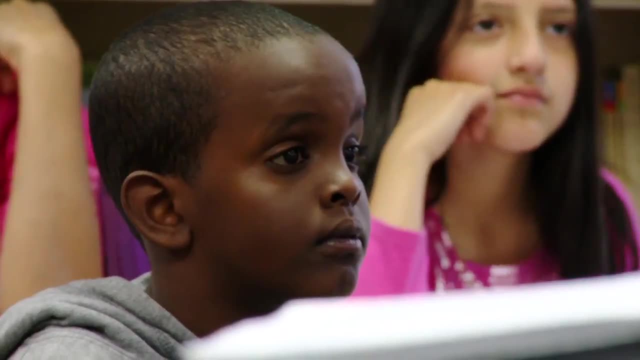 We will make decisions with our partner about how to count the number of objects in a collection. Nice job. Counting collections helps students to learn different ways to count rather than just counting by ones, Counting in ways that are more efficient, maybe by fives, tens, twenties. 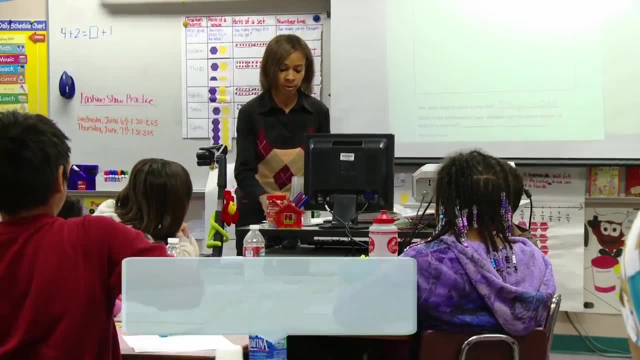 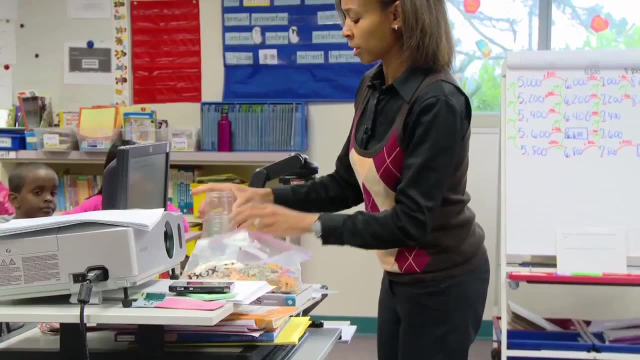 So I want to first show you some ways that you might count your objects. So here are some cups and here's my puzzle pieces. My partner and I can decide the best way to count these. So I might decide to put them in groups of ten. 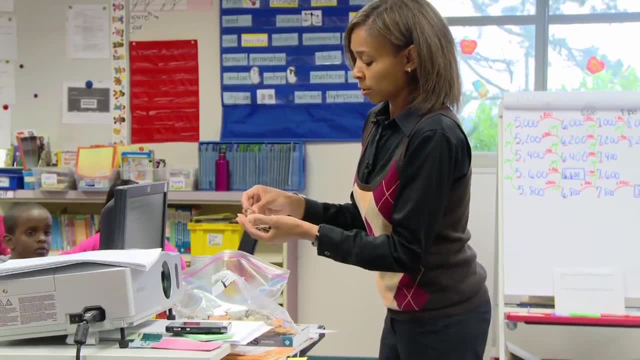 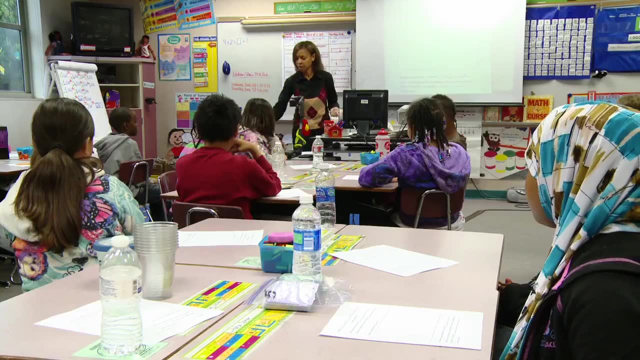 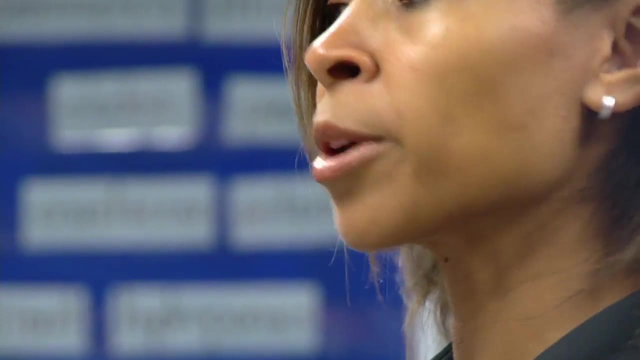 So I'm just going to count by twos, Two, four, six, eight, ten, And then I'm going to put that cup to the side because it's done, And then, after I have all of my cups, that's when I, me and my partner and I 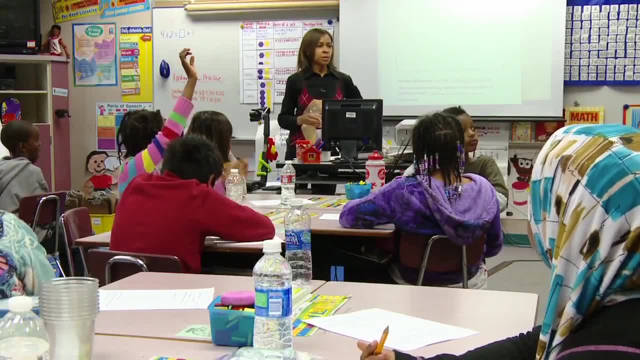 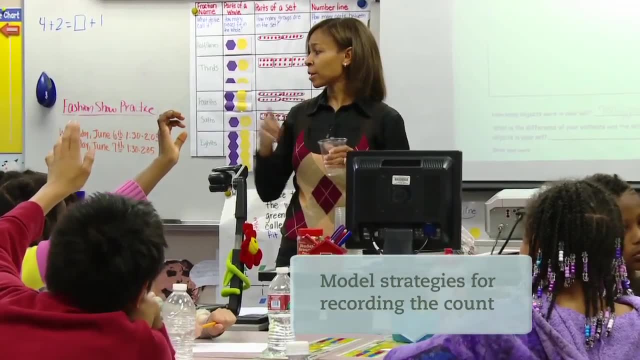 we'll count them. What are some ways to record this? Like if I just group all of these in groups of ten? what are some ways I could record it? Can you quickly come show us up here? How would we record if I group all of those puzzle pieces? 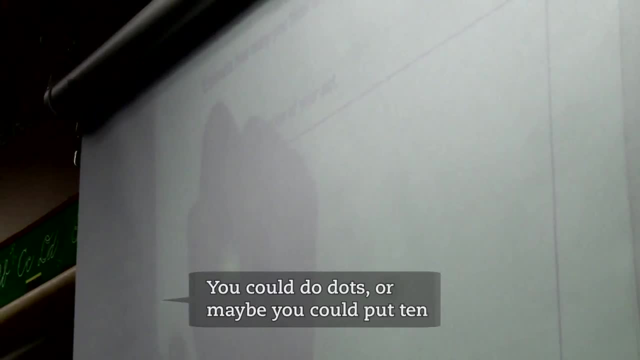 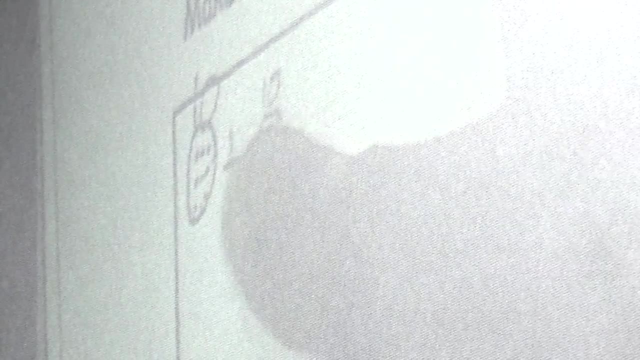 Wait, so you count it by tens, I count it by tens. yeah, You could, you know, just do dots, or maybe you could just put ten and then a plus sign. So Areli said, you could either do ten dots in a circle. 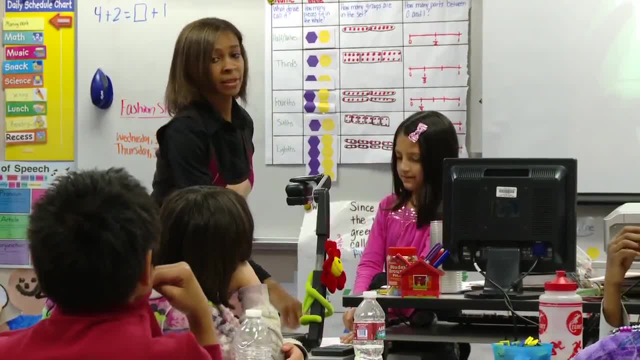 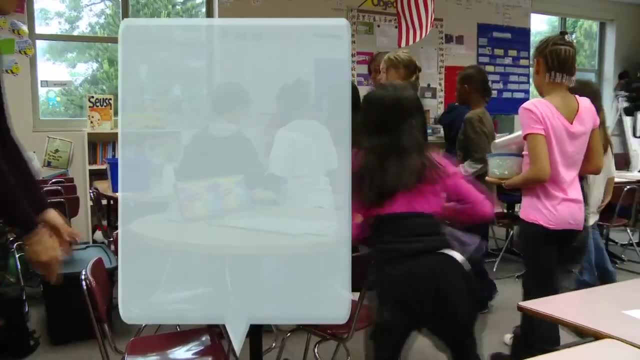 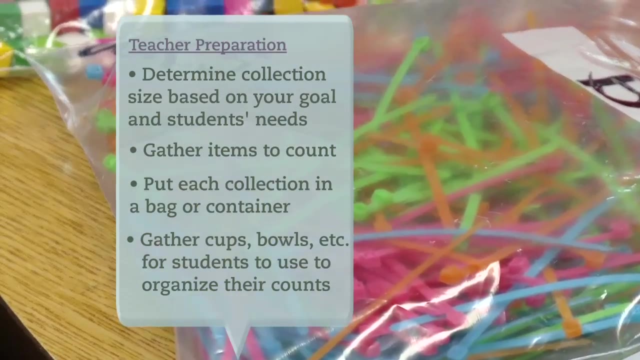 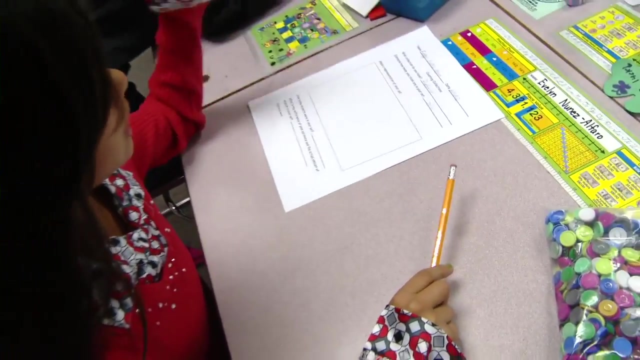 or you can just put a circle and label it: ten plus ten plus ten until you get done. Yeah, Any questions about that? All right, Okay, you guys can get your collections Two thousand Fifties, Fifties, just like we said. 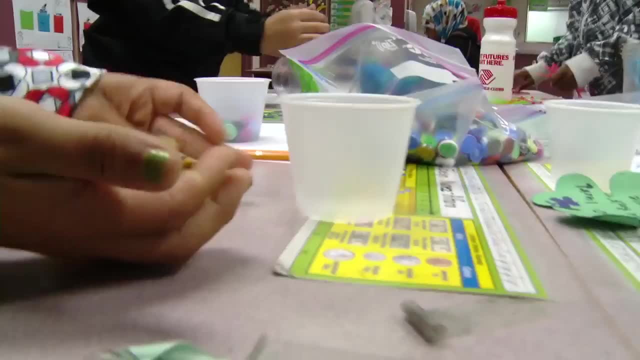 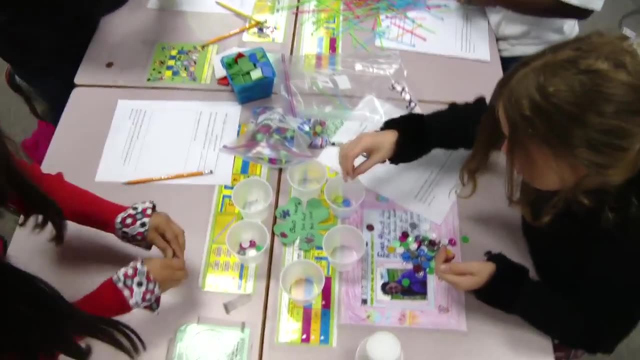 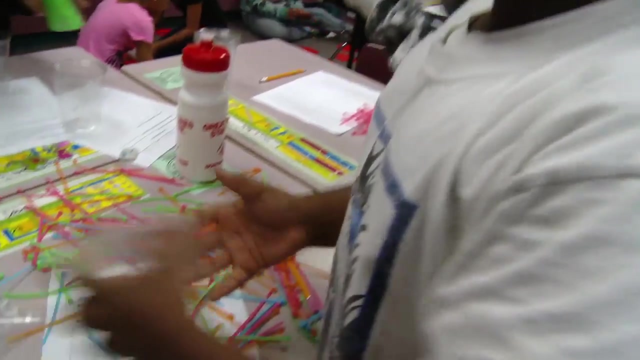 So just grab a handful and try to fit fifty in one, Thirty-two, thirty-one, four, One, two, three, four. We have our own colors and we count, and then we try to add fifty in each cup And then we're going to count them by fifties until we get our answer. 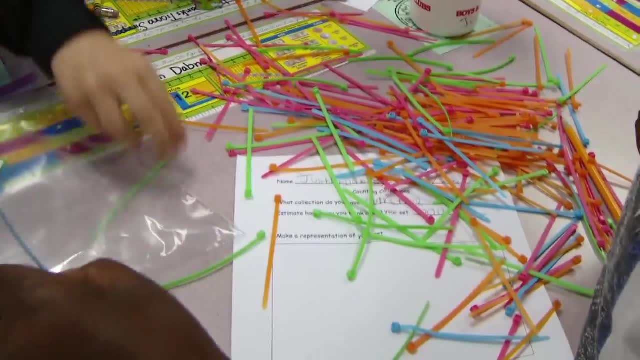 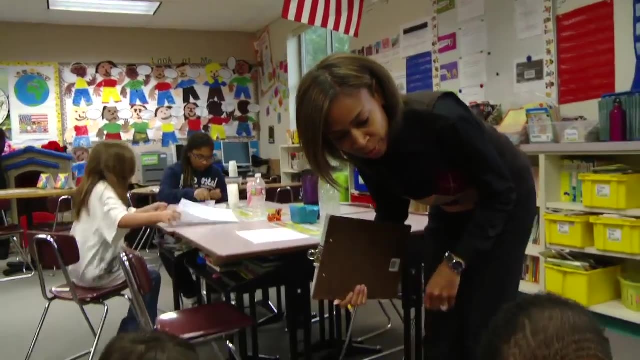 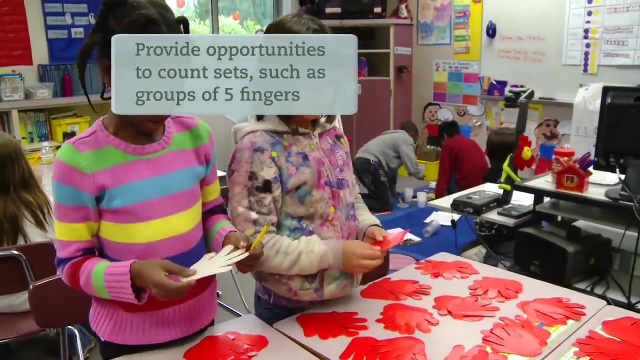 One, two, three, four, five, six, seven, eight. Have you guys made a decision on how to group them? How are you grouping them? Fifty, Fifty-two, Wow, fifties. While my students are counting their objects in their collections. 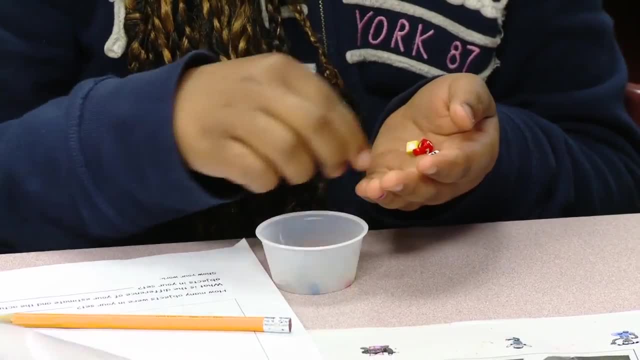 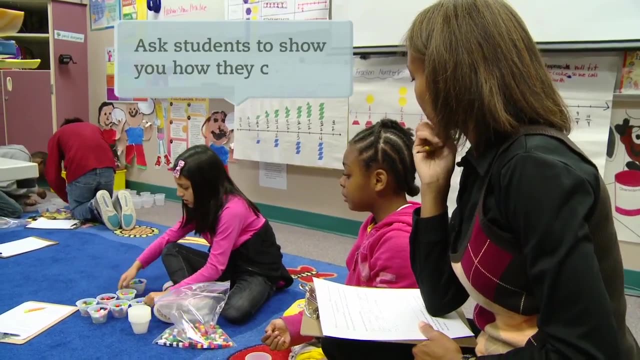 I'm walking around looking at students and how they're grouping their objects, how they're keeping track of their objects, the ones they've counted, making sure they're not counting them twice When you put them in your cup. how are you counting them? 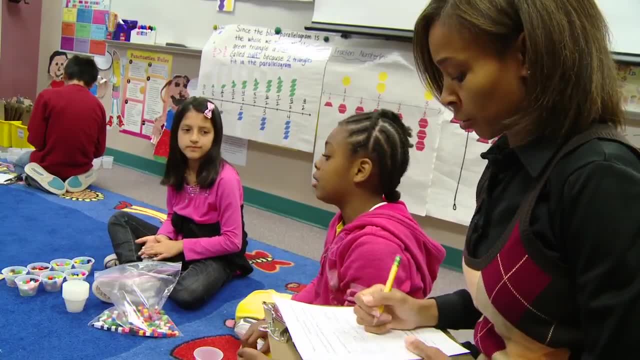 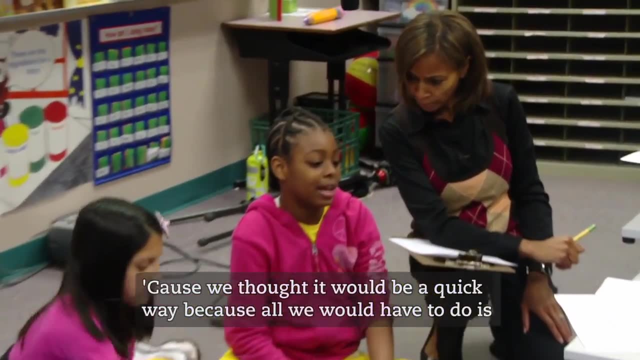 Are you saying one Fifty in each cup, So you're putting them in groups of fifties. Yes, Why are you putting them in groups of fifties? Because we thought it would be a quicker way, because all we have to do is be at fifty one hundred. 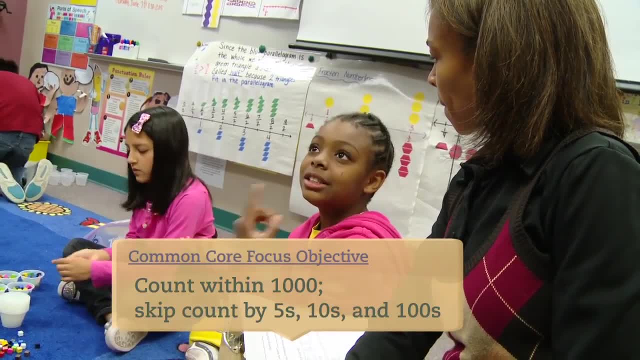 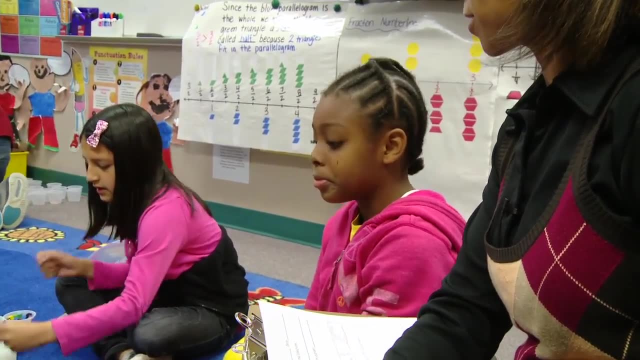 and then you add fifty, two hundred, two hundred, fifty, six hundred, three hundred, and it'll be a more efficient way, More efficient way. So if you're counting by fifties, Mm-hmm, How are you guys grouping yours? 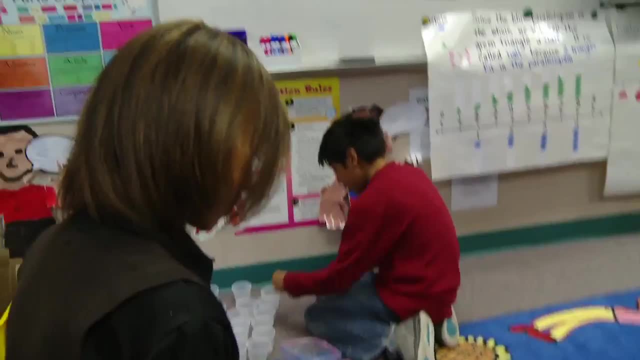 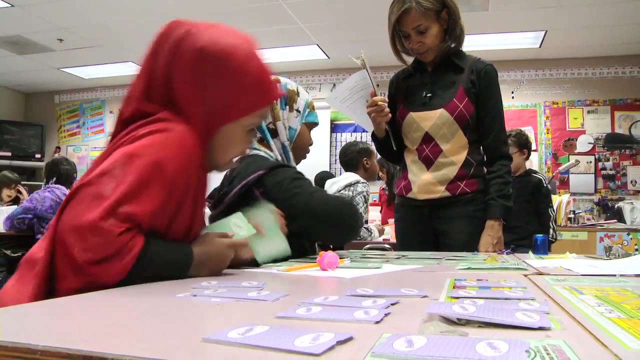 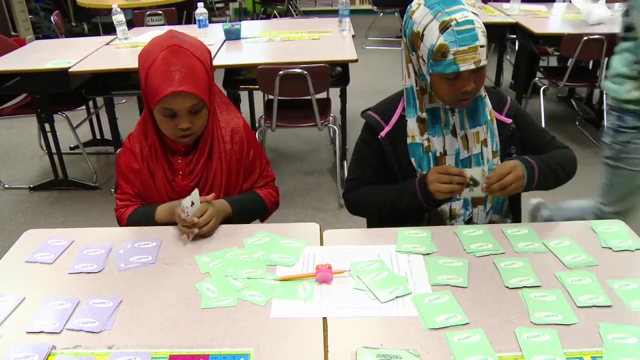 By tens. By tens, You have to be able to work well with your partner. to be successful at counting collections, You have to be able to agree on a way to count. I saw two of my girls. They had green cards and they had purple cards. 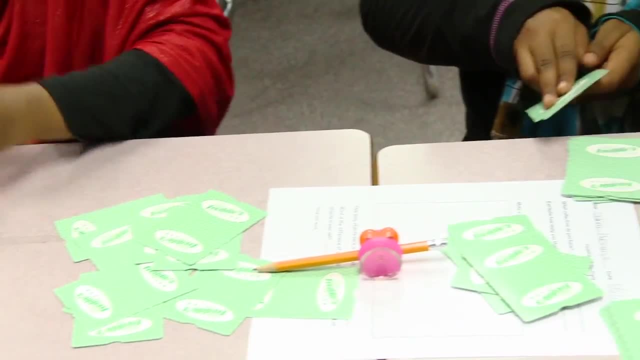 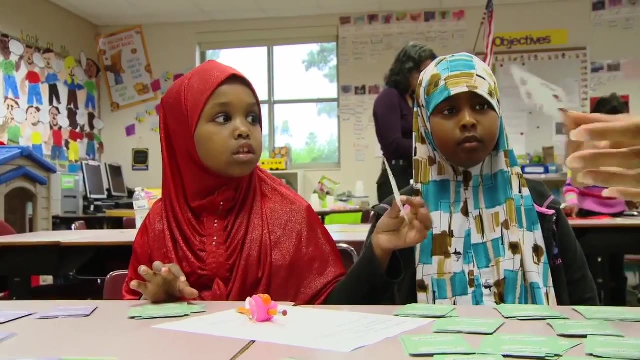 And so they shared the responsibility. One girl would count the purple cards and another student would count the green cards. Is that a group of ten, Mm-hmm? And then what do you have? Two leftovers. So what should we do with these two? 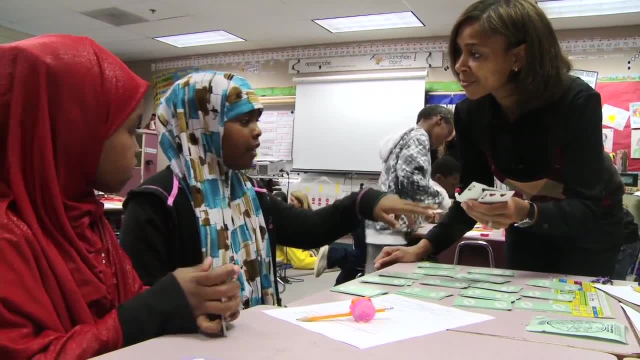 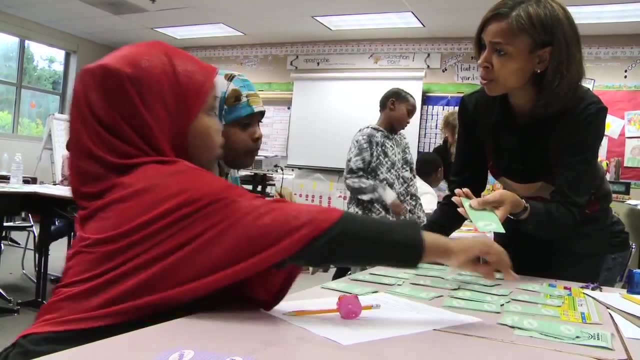 She has eight and this is two. So eight plus two. So eight plus two is ten. Wow, So what could we do with this? eight plus two is ten. What could we? We can put them together, Mm-hmm. 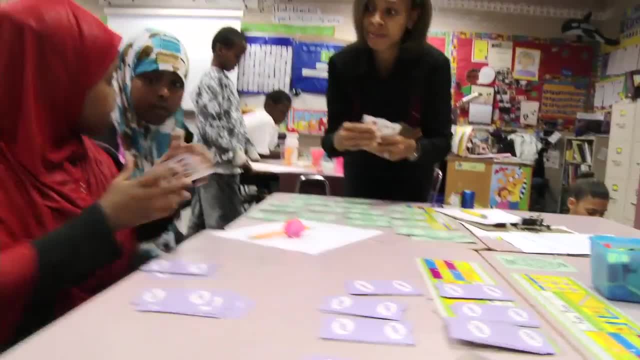 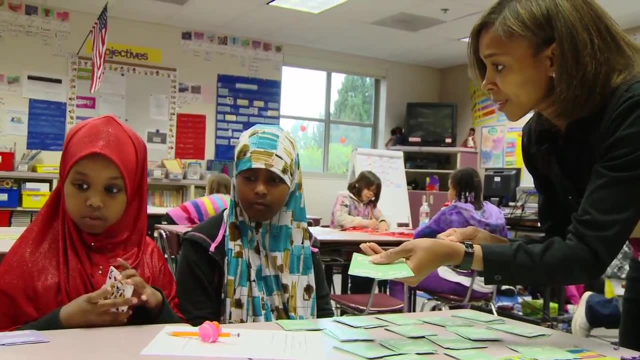 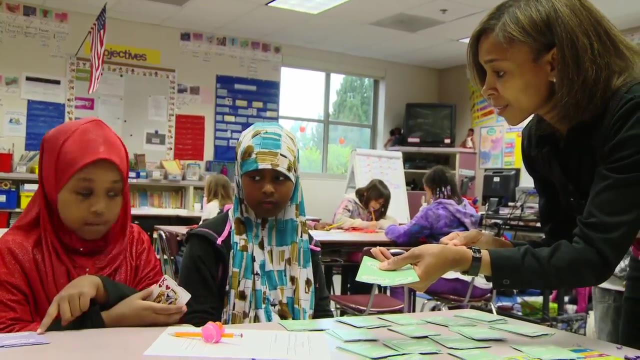 Okay, Where is the eight Here? Is that your group of eight? Yeah, What should we do with these, Sarah? We should do that when we should count the tens, and then we should make these two last. Wherever number will land on, we're going to count by ones. 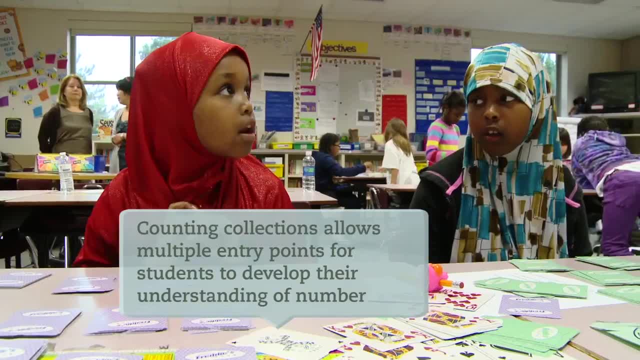 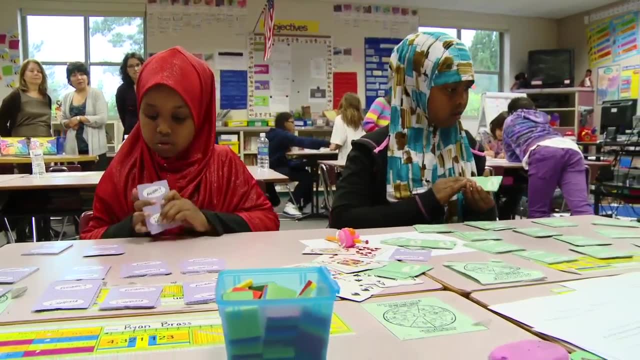 Okay, So you're different strategies, but both of them are correct, So I'm going to let you guys decide which one you're going to do. All right, Awesome. So I would say, just keep these out of the way, so you'll know. 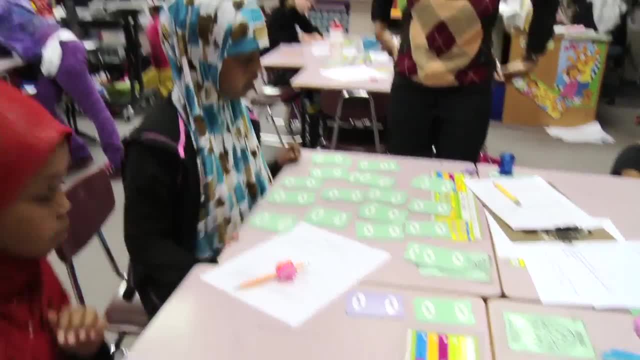 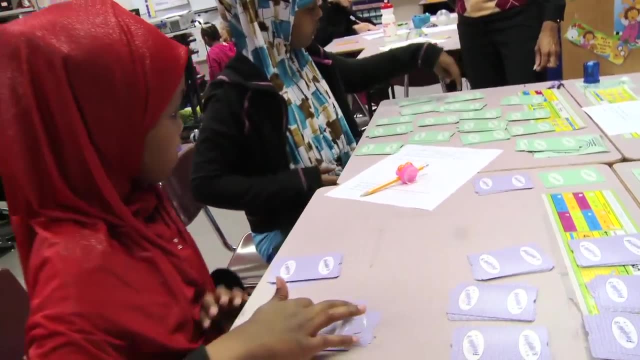 And then go ahead and count your cards: 10,, 12,, 13,, 14,, 15,, 16,, 17,, 18,, 19, 20.. Students are understanding how not only to count, but they're also learning how to record. 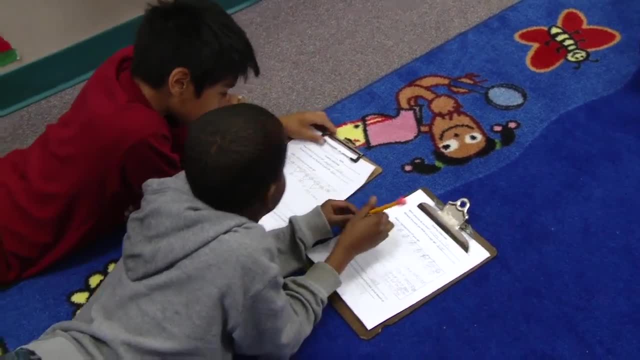 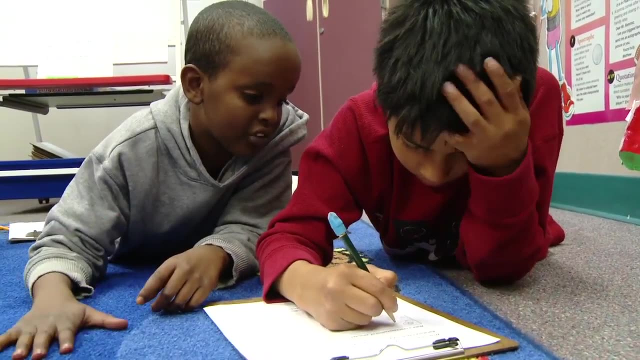 And how to add their collection. Okay, Now draw a circle And put 50.. Draw nine of those And then add the last one. There's 79.. So 50. And now add 50 plus 50. Equals 100. 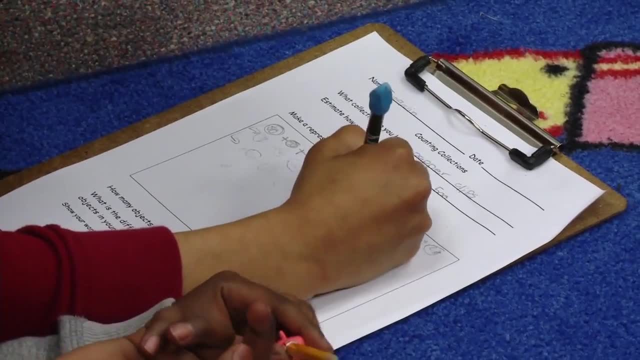 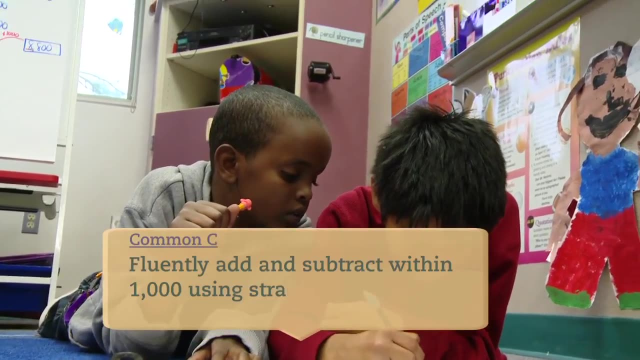 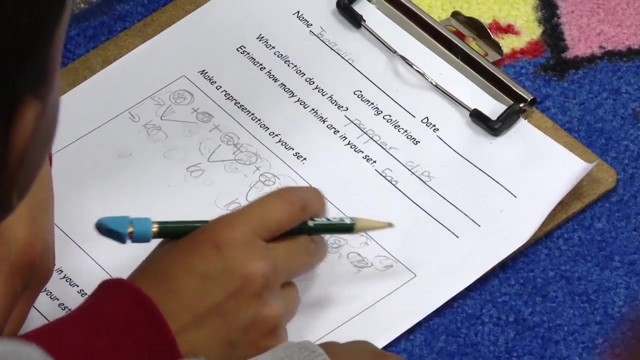 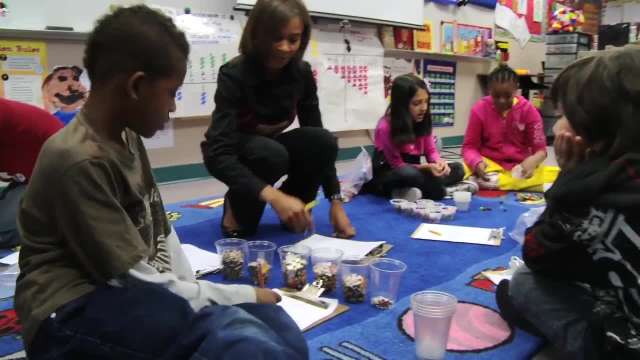 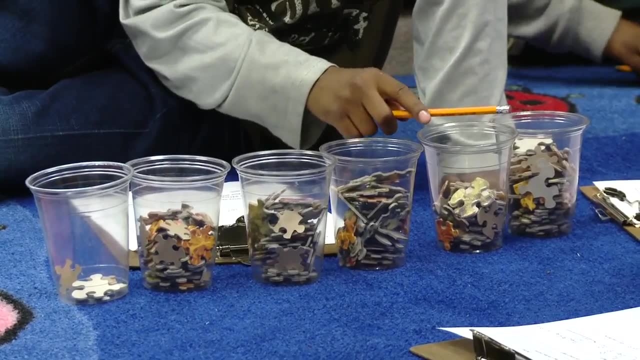 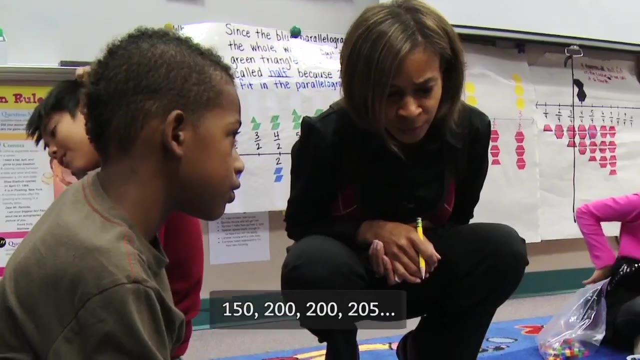 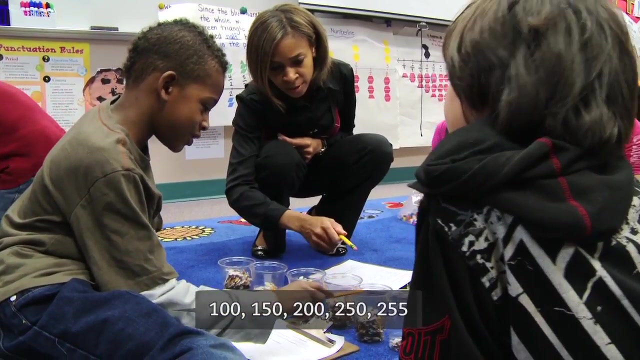 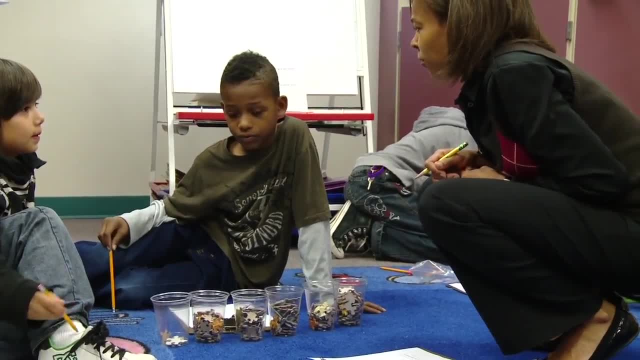 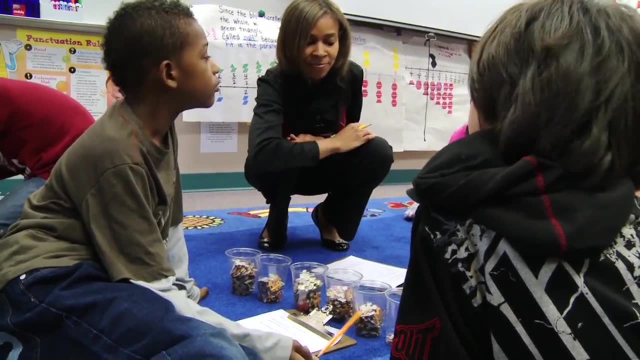 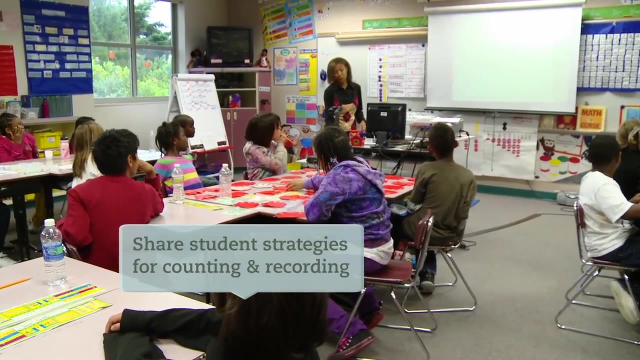 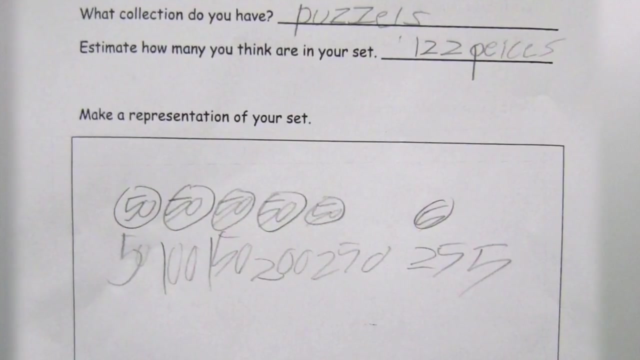